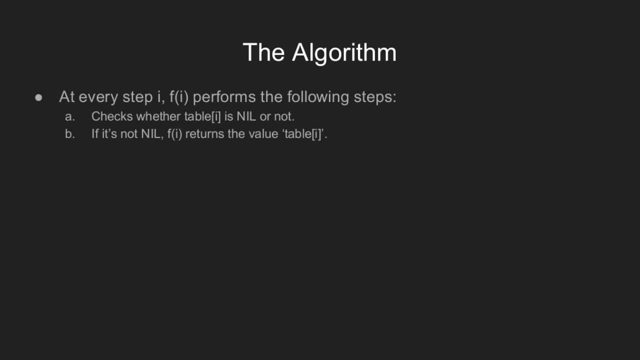 At every step i fi first looks into the lookup table to check whether a solution is stored there. If a solution is stored, that is, table i is not nil, fi returns table i. If a solution is not stored, fi checks whether i satisfies the base condition. 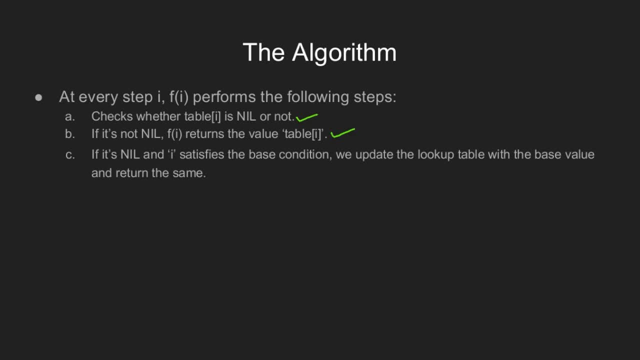 If it does satisfy the base condition, we update the lookup table with the base value and return. However, if i does not satisfy the base condition, then fi splits the problem i into subproblems and recursively calls itself to solve them. After the recursive calls return, fi combines the solutions to subproblems. 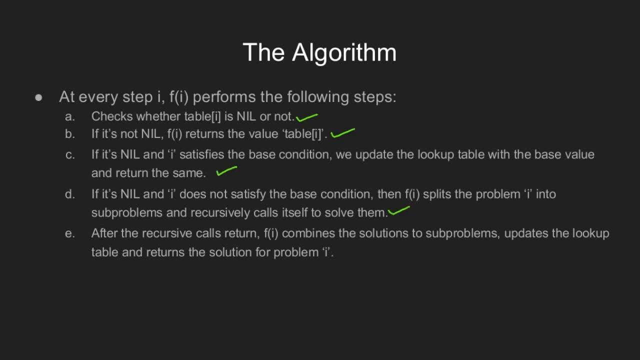 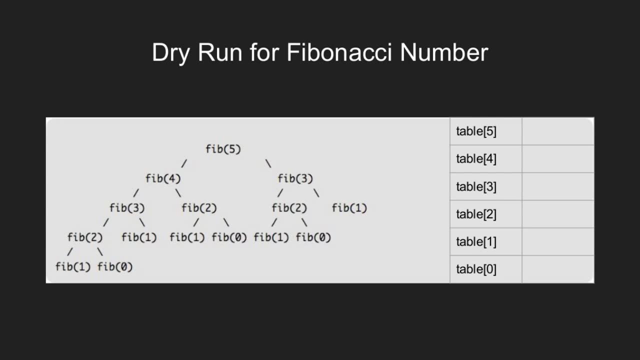 updates the lookup table and returns the solution for problem i. Let us see how memoization will work for our Fibonacci number problem that we discussed earlier. First we initialize all the entries in the lookup table as nil. Next we call Fib5. But table 5 is nil and 5 does not satisfy the base condition. 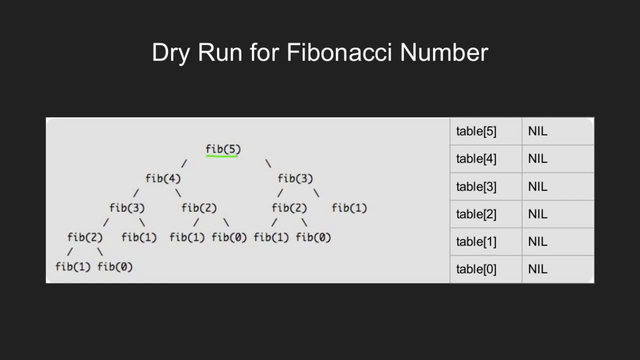 So Fib5 splits the problem and calls Fib4.. Now control moves to Fib4. But again table 4 is nil and 4 does not satisfy the base condition either. So Fib4 splits the problem. This goes on until we reach the base condition, Fib1.. Now Fib1 updates. 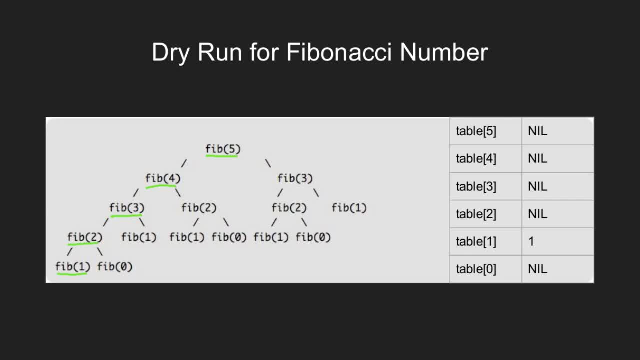 su2 and returns 1.. Then control goes back to Fib2, which in turn calls Fib0. And similar to Fib1,. Fib0 updates table 0 with 0 and returns 0.. Once again, control moves back to Fib2,. 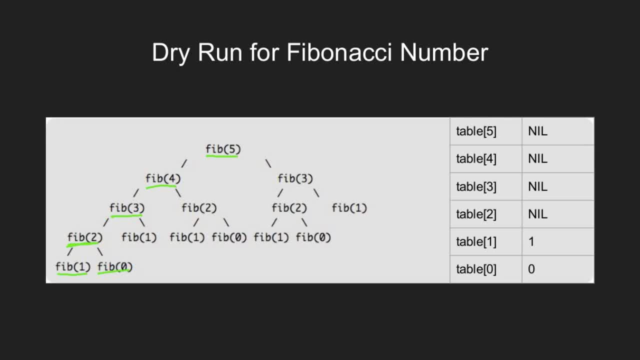 which now combines the solutions of Fib1 and Fib0 and stores the result in Table2.. Now contrast: on page 116, control moves back to Fib3, which in turn calls Fib1. However. However, this time table1 is not nil, so fib1 simply returns the value stored there. 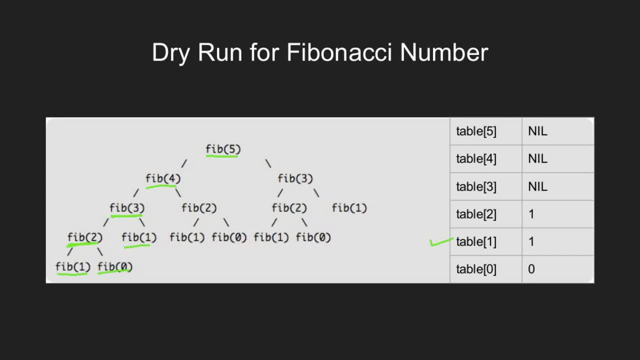 Consequently, fib3 combines the solution to fib2 and fib1 and stores the result in table3.. Now we move up to fib4, which calls fib2.. Since table2 is not nil, fib2 simply returns the value stored there. As a result, fib4 updates table4..